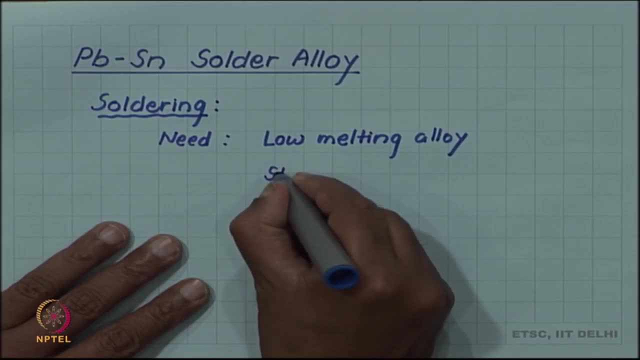 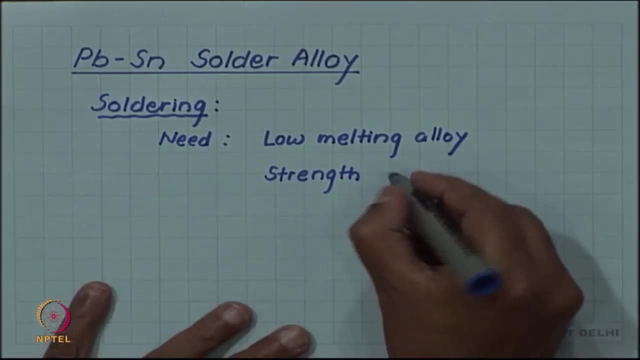 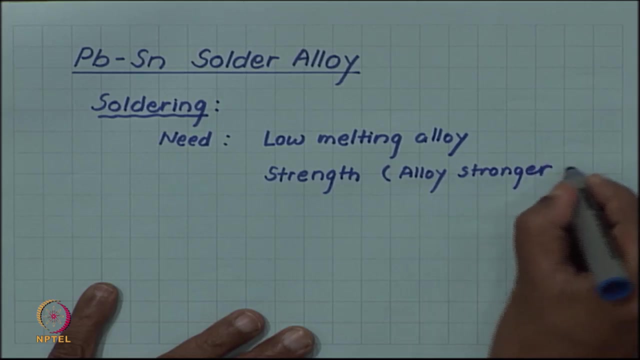 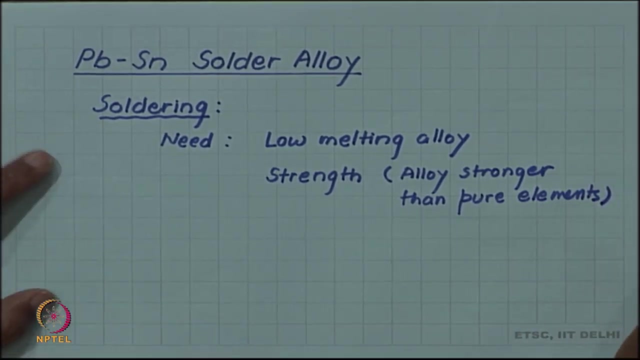 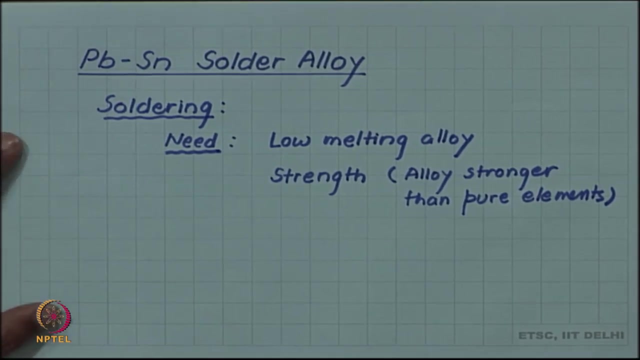 or a pure element, because you also need a strength And you will see during in this course, the development of this course, that alloys always have better strength than pure elements. This is general rule. this is called solid solution strengthening And we will have more time to discuss that later in the course. So lead tin makes a 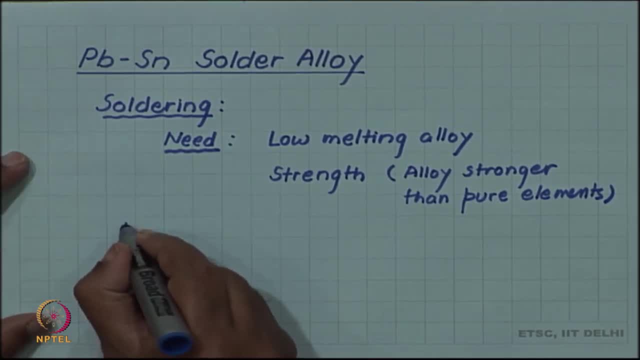 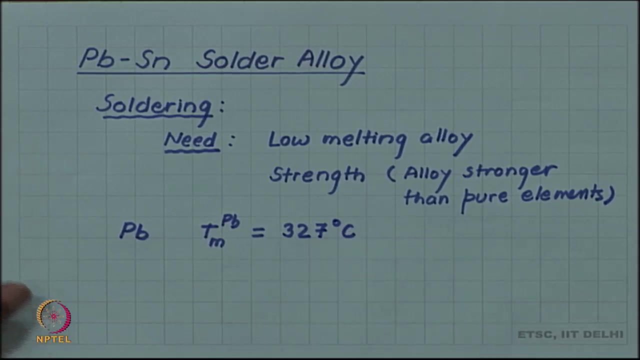 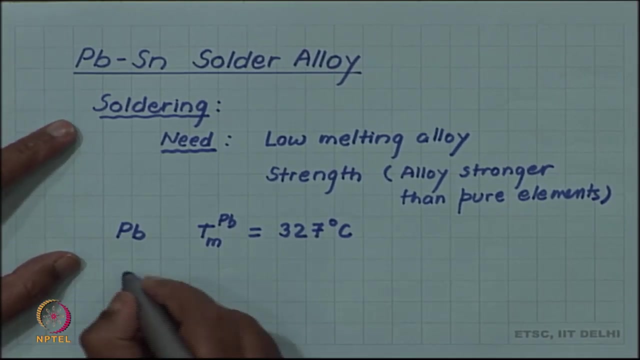 nice candidate for this, because lead itself has a melting point of 327 degree Celsius, which is reasonably low. If you compare it with your previous example of copper and tin, which were both having more than 1000 degree Celsius as their melting point, lead has only a melting point of 327 degrees Celsius. 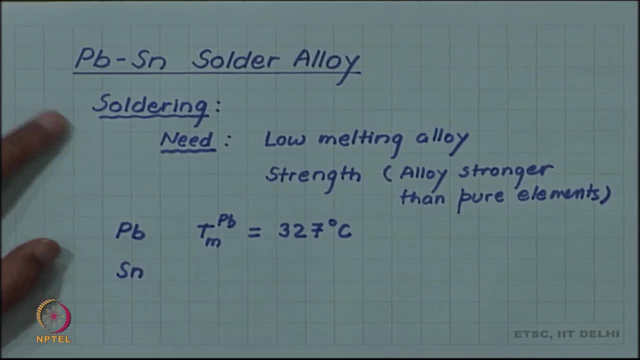 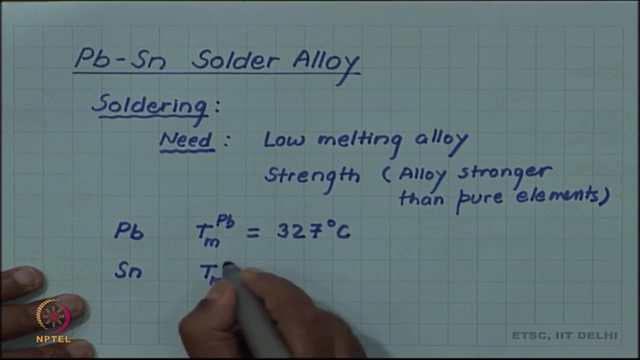 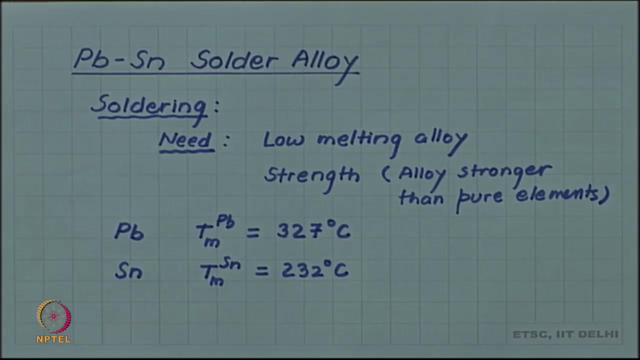 And still to strengthen it, we have an alloying addition And we select another alloying addition which is even lower melting point. So the melting point of tin is only 232 degree Celsius. So hopefully, since we are adding a lower melting point, alloy in a higher melting point. 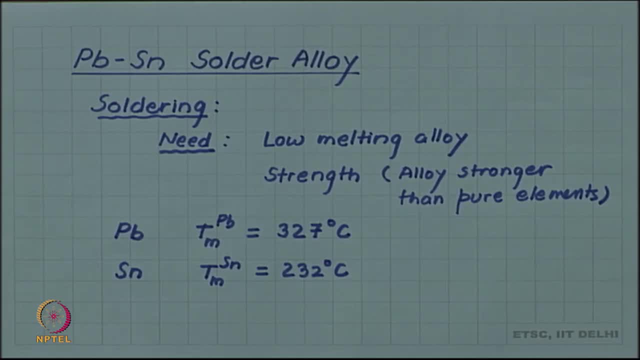 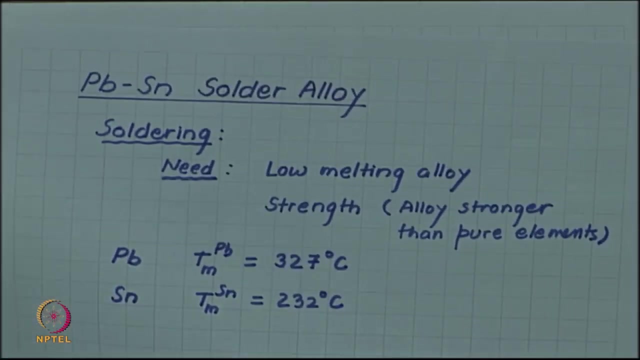 system. probably we will get an alloy which may have even lower melting point, which will be even better from the point of view of soldering, because you want to heat it, to melt it, and this heating will be easier, or melting will be easier if the melting point is low. 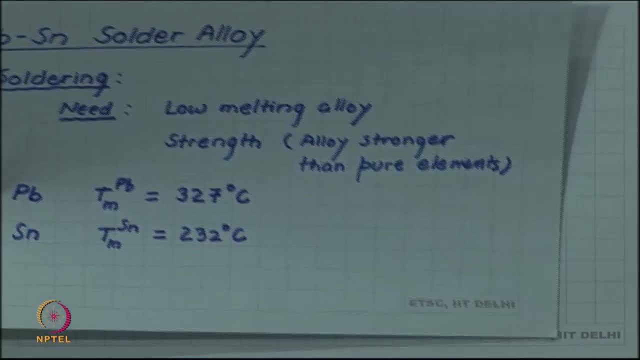 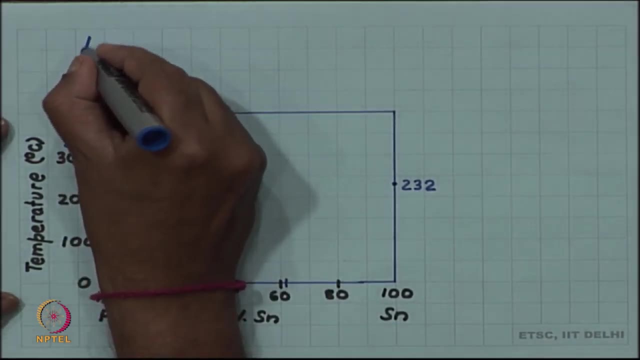 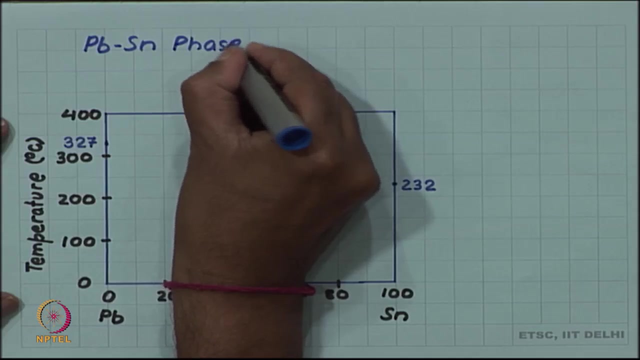 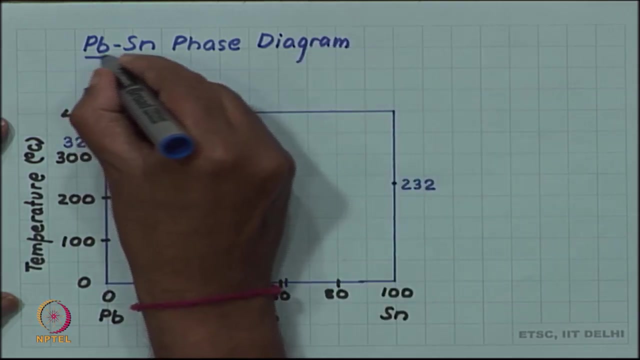 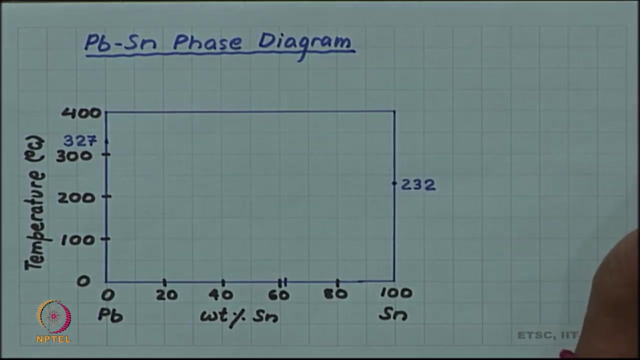 So let us look at what the lead tin phase diagram looks like. So here I am going to draw a lead tin phase diagram for you. You are now familiar with this. In this box for our binary alloy, the x axis is components. so, since it is a lead tin alloy, 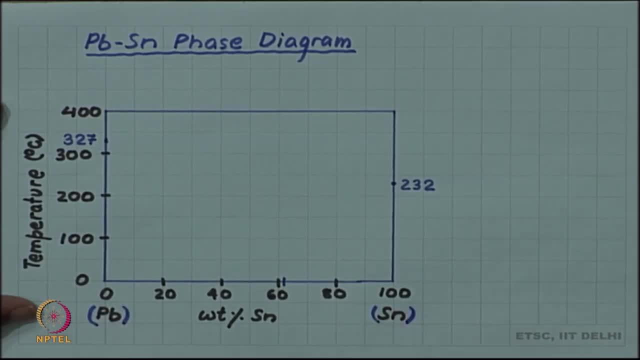 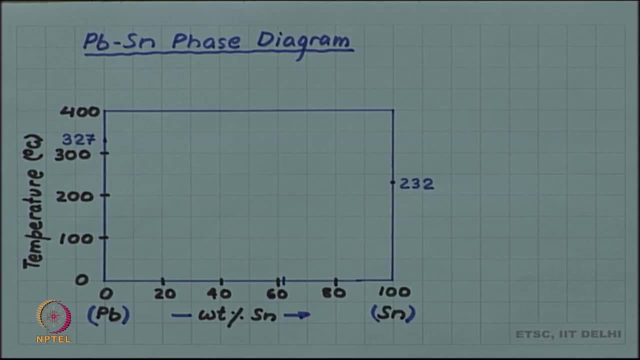 so the components are lead and tin and we decide to use weight percent tin as our x axis. So, since it is a lead tin system, 0 percent tin denotes lead, 100 percent tin denotes pure tin. So here is our temperature axis. 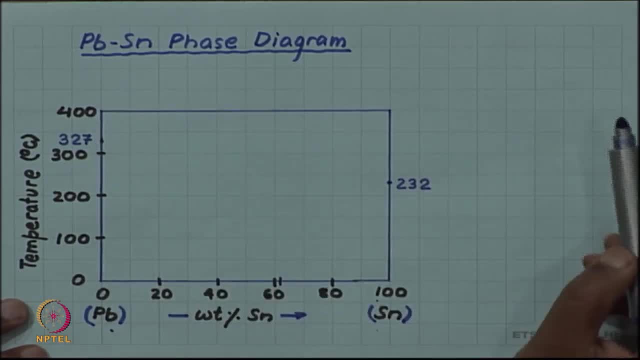 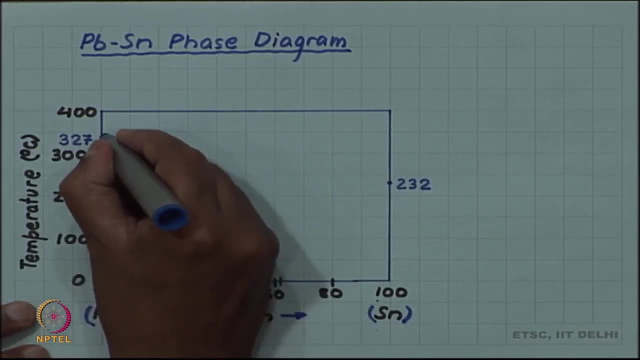 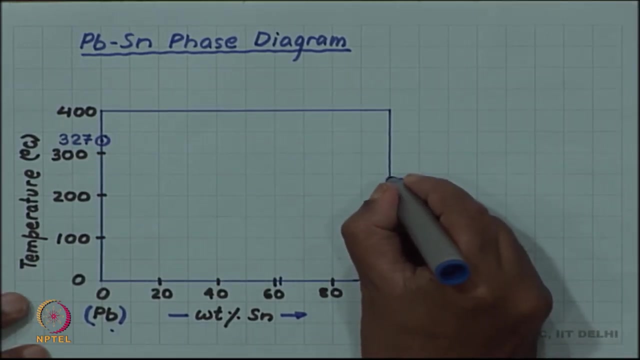 Now we do not have to have temperature axis running in to 1000 degrees Celsius, highest temperature, the melting point is only 327, that is of pure lead. So we have that on the lead axis and we have 232, which is the melting point of tin on. 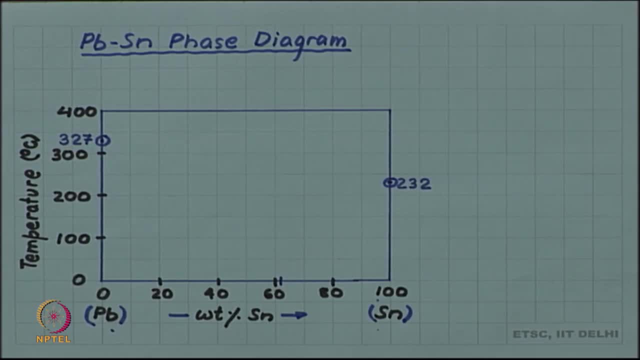 the tin axis, And you have already seen 5 dreadών.0100103it2209يرة08 hides. 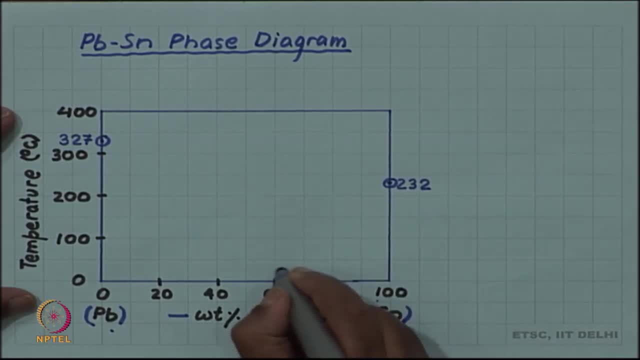 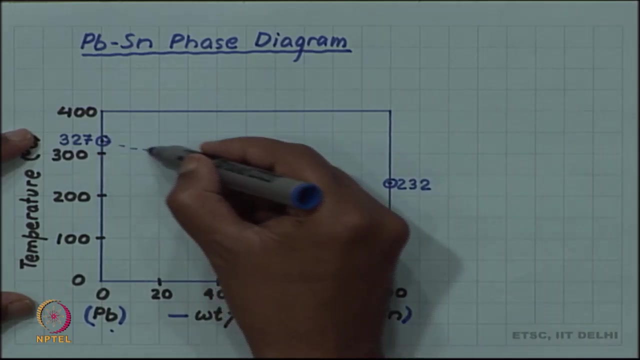 Let us say: if we want the melting point of alloy of 62 weight percent- you will soon see why I am selecting something odd like 62, but suppose I want a melting point of 62 weight percent in alloy- Then we have already seen that our first approximation, which was a linear approximation, was not 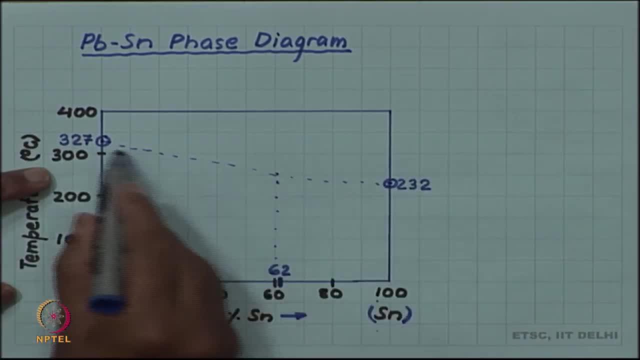 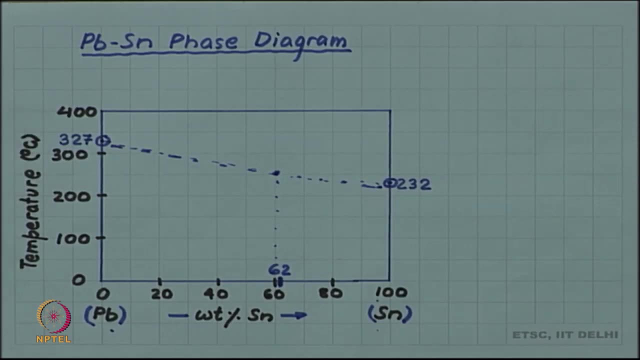 very right. my line is not very straight, so excuse me for that. maybe I will try something better this time. So if I draw a straight line and if I try to predict a melting point, I get something close. But that is not the truth, because now you know better that for alloy, the melting point 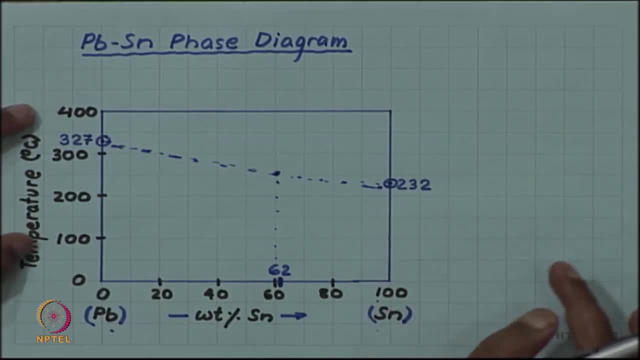 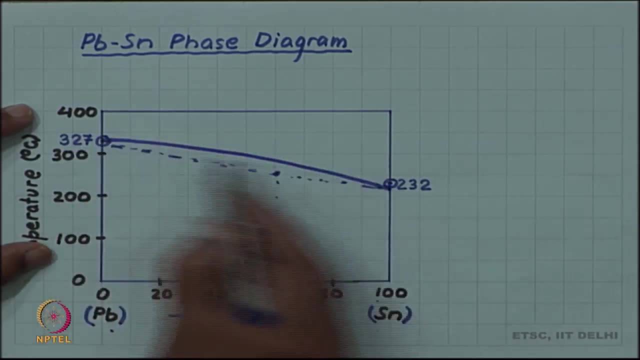 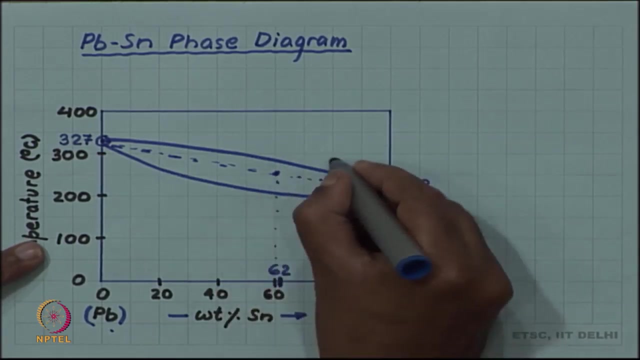 is not happening at, or melting is not happening at, one unique temperature but over a range of temperature. So you saw in the copper nickel diagram that there was a liquidus and a solidus. so you can predict something like this that you here also, you will have a liquidus. 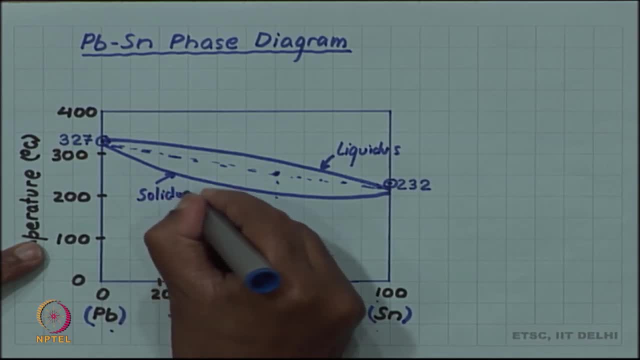 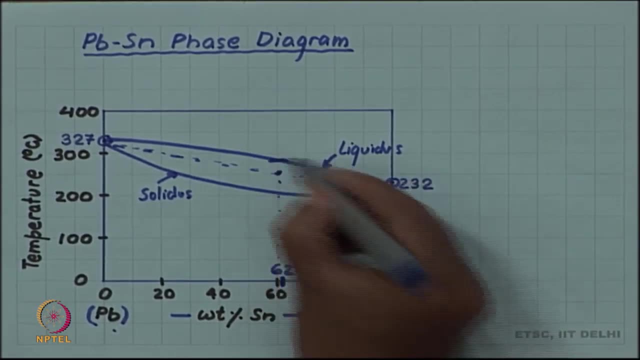 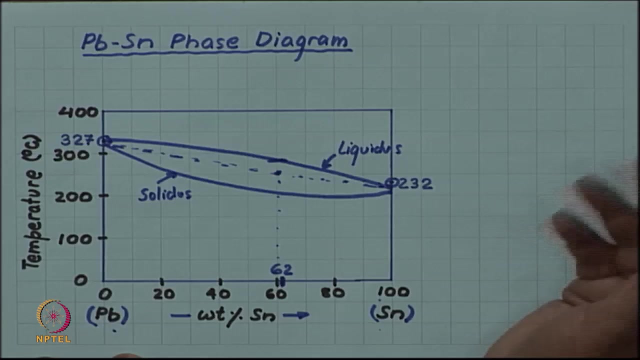 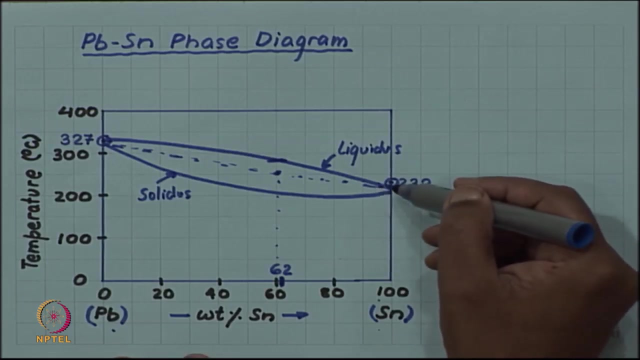 And a solidus, and this gives you an alloy which will melt at a lower temperature than the higher melting component, lead, And this is intuitively obvious because we are adding tin. so we are, we were thinking that we are adding low melting component to a high melting component, and that is bringing 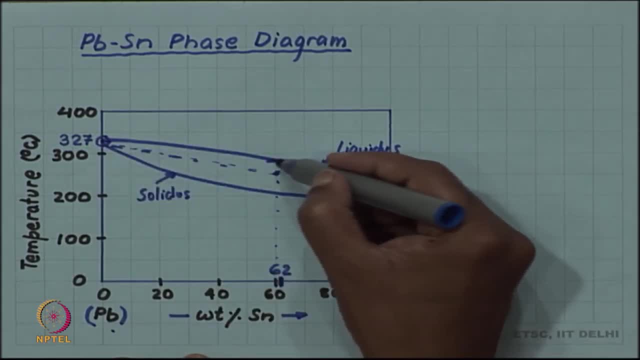 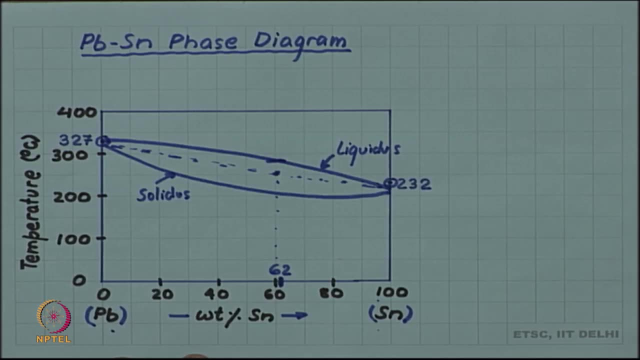 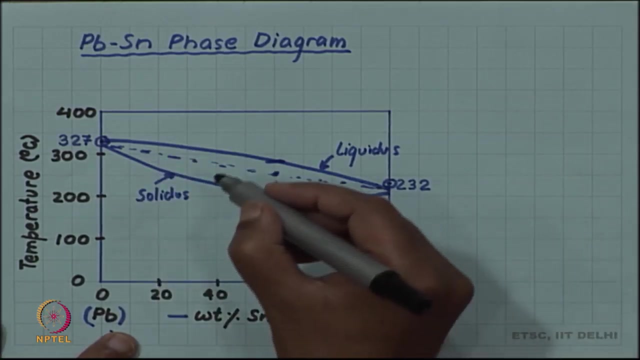 down the melting point from 326.. Okay, From 327 to somewhat lower temperature. however, in reality, you get a even better result. you get more than your expectation And the liquidus is not a continuous line like this in the lead tin system, if you see. 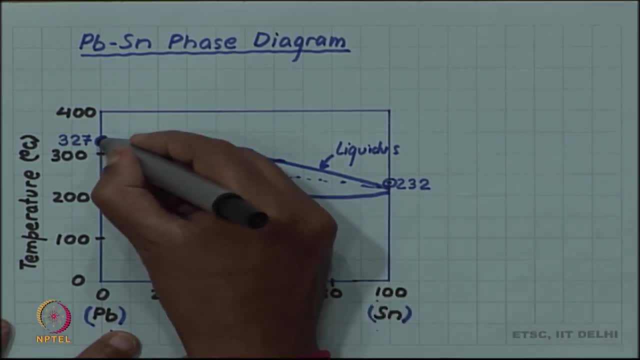 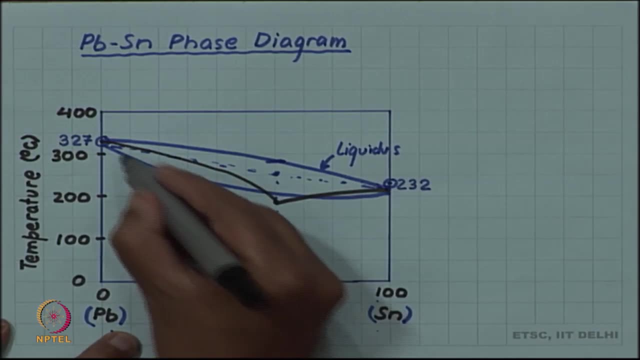 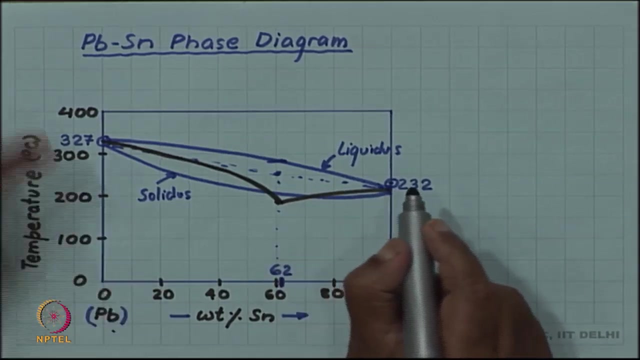 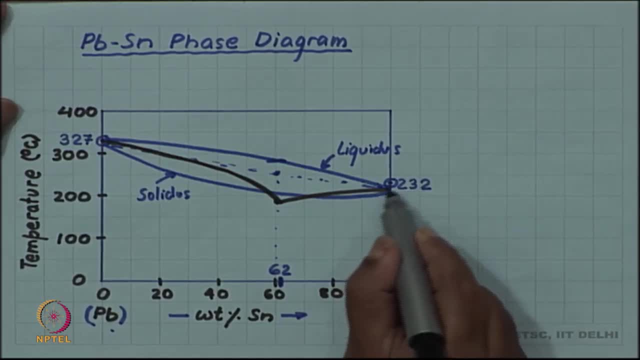 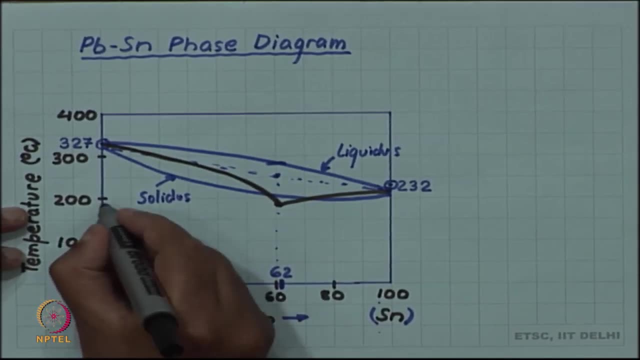 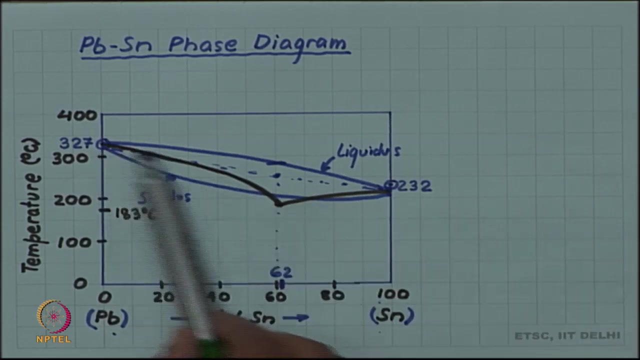 melting point of lead and one is starting from the melting point of tin And both converging at to a minimum point, which is 183 degrees Celsius. So this is very, very interesting. This is very interesting. Okay, this is more interesting than a continuous liquidus like that. 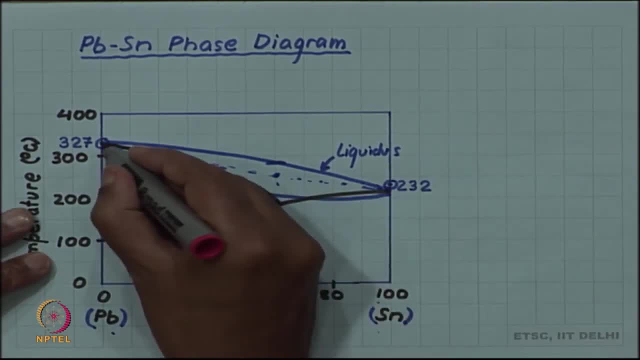 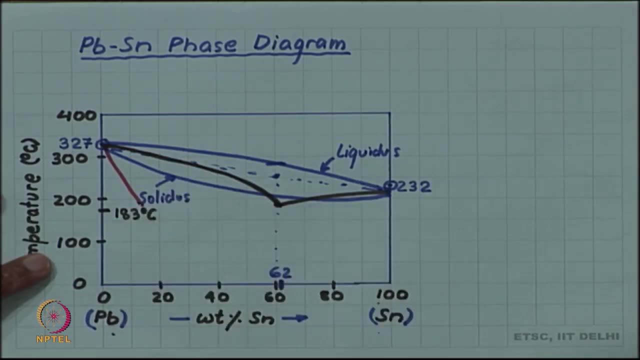 And what does the solidus do? Solidus also makes an interesting turn and solidus actually breaks into two different solidus. instead of a continuous solidus, Now you have two different solidus and they end at that same temperature of 183 degrees Celsius. 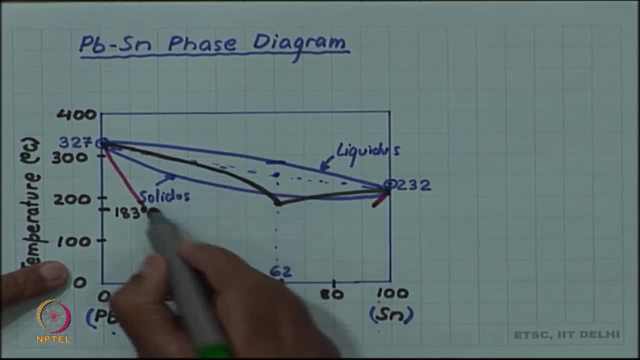 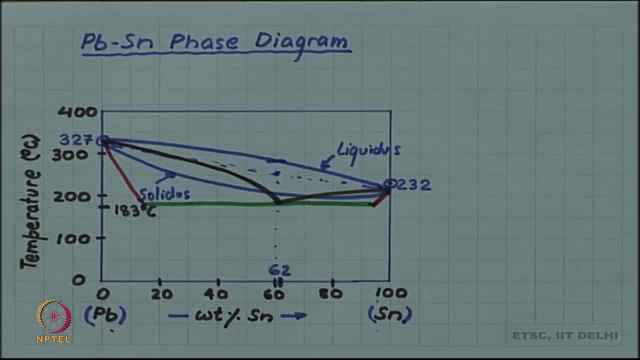 And then, at 183 degrees Celsius, you have a horizontal line going through this minimum of the liquidus from one solidus end to another solidus end. And finally, to complete the phase diagram, You have two more lines, two new lines which you have not seen in an isomorphous diagram. 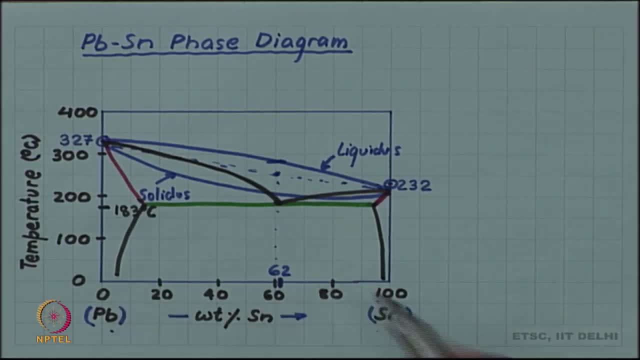 extending from this end to this end. So you can see this is a somewhat more complicated but at the same time more interesting phase diagram than the simple isomorphous diagram. So since the earlier isomorphous expected, The first expectation is superimposed on this and is confusing the diagram. let us look. 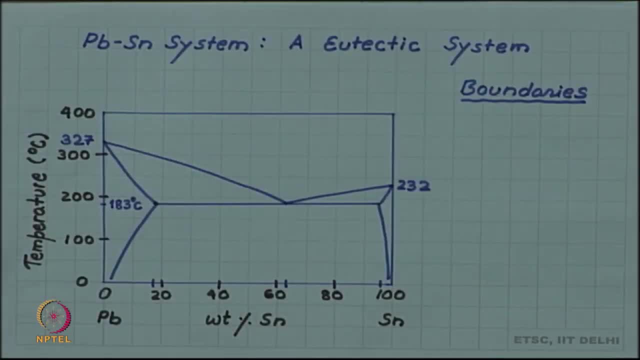 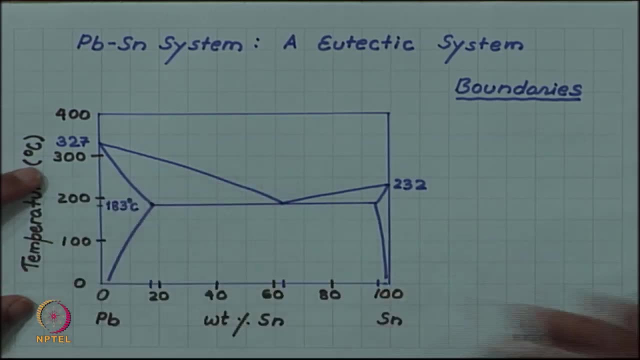 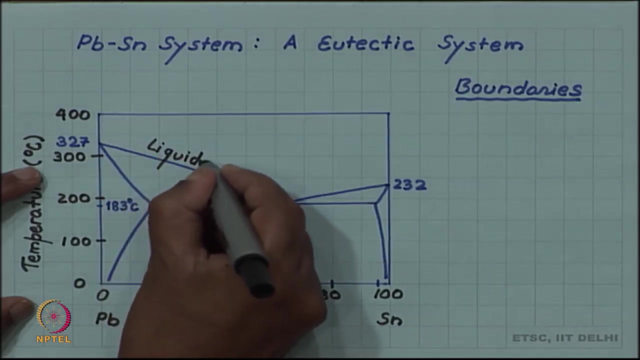 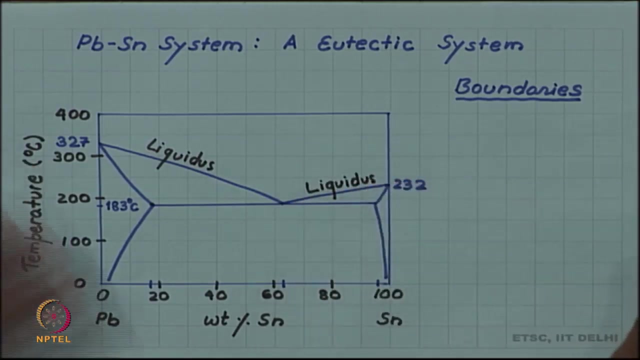 at the diagram in its own. So what we have seen is that you have liquidus in two components, So let us write down those boundary names. So you have liquidus We have not yet divided. Okay, We have defined liquidus, but we can do that. 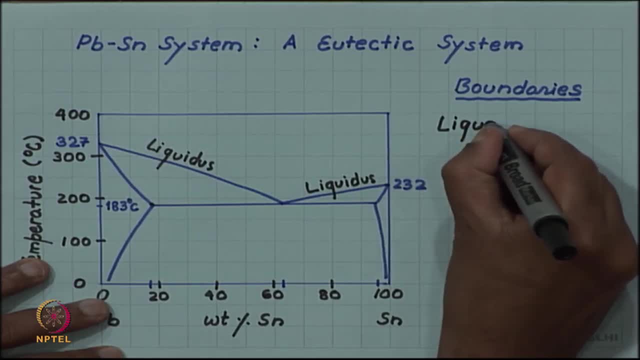 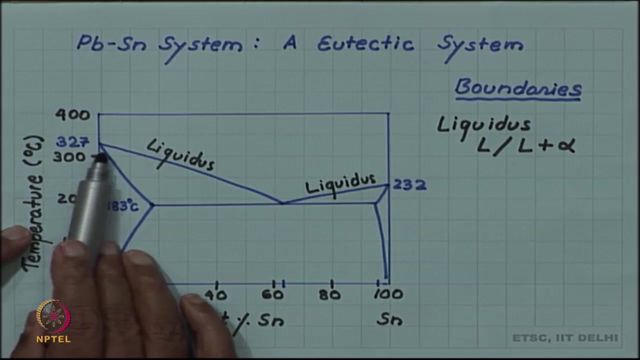 So liquidus is any boundary which separates a single phase liquid with a mixture of liquid and solid. So this is a liquid, liquid plus alpha phase boundary, this is liquid plus liquid liquid and liquid plus beta phase boundary I have not yet mentioned. 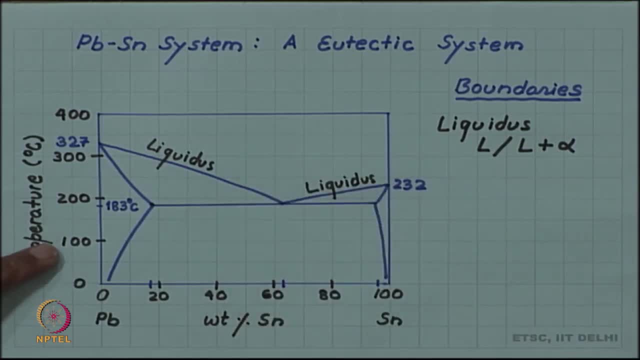 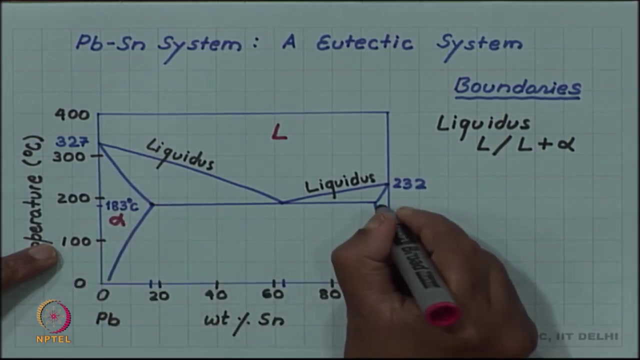 The phases. So let me first label the phases in this diagram. So above the liquidus you have liquid. These two end triangular regions are solid phases and now you have two distinct solid phases. So unlike isomorphous diagram where a single phase was extending from one end to the other, 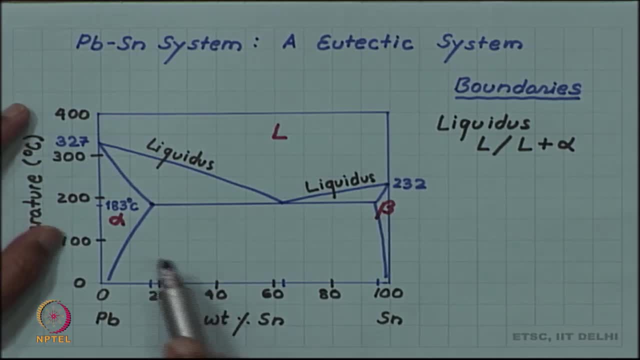 end. Now you have Two different solid phases in the same alloy system. So near the lead end you have a alpha solid phase and near the tin end you have the beta solid phase. These are the single phase field and if you apply your lever rule you will get other two. 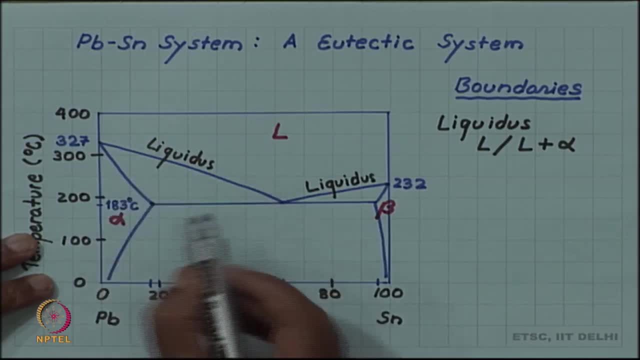 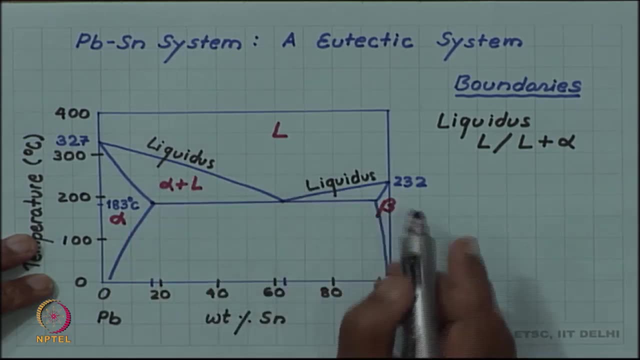 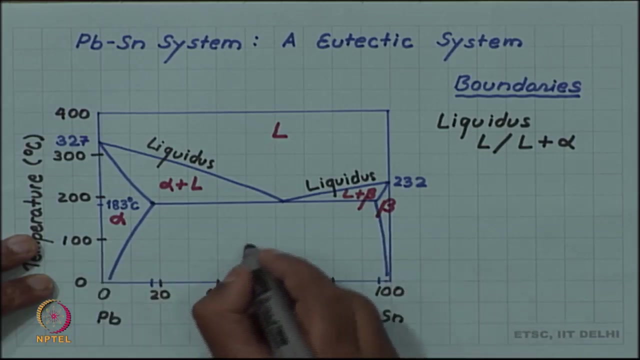 phase regions here. So you can see here one end alpha, another end liquid, So this is alpha plus liquid region. Here one side liquid, another side beta. So this is liquid plus liquid, So this is liquid plus beta region. and here one side alpha, one side beta. 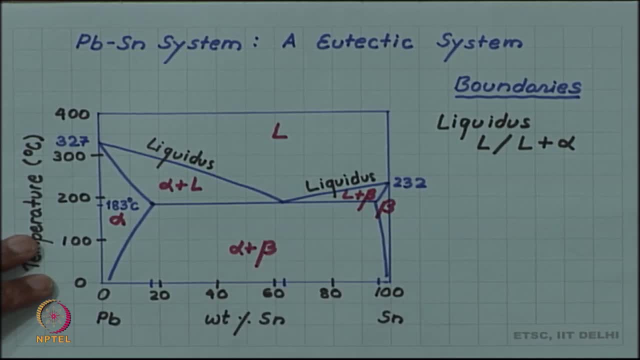 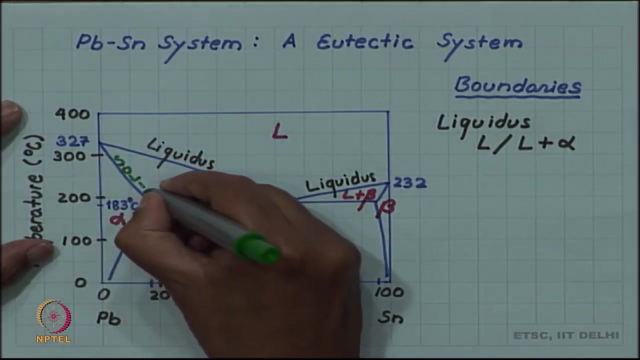 So you have alpha plus beta region. So all the phase fields are labeled, and now I am labeling the boundaries for you. So this is the liquidus boundary, These boundaries are the solidus. So this is solidus and this is also solidus. 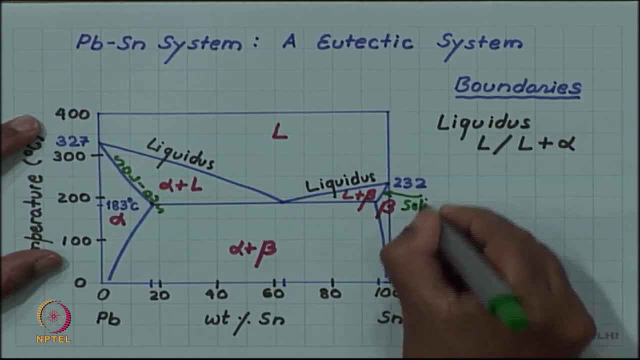 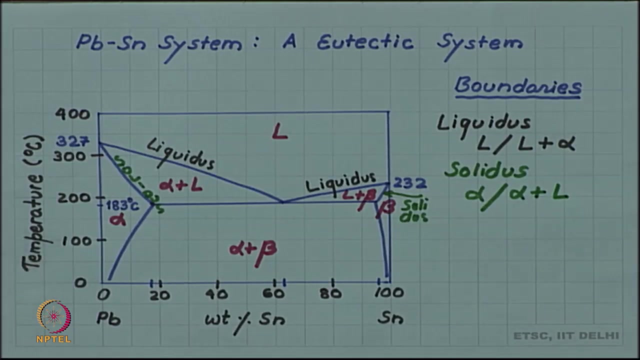 So this is solidus, So this is solidus. So solidus is a boundary between a single phase- solid and solid, plus liquid phase to any boundary. So we had seen liquidus and solidus in the isomorphous system, the copper nickel system. 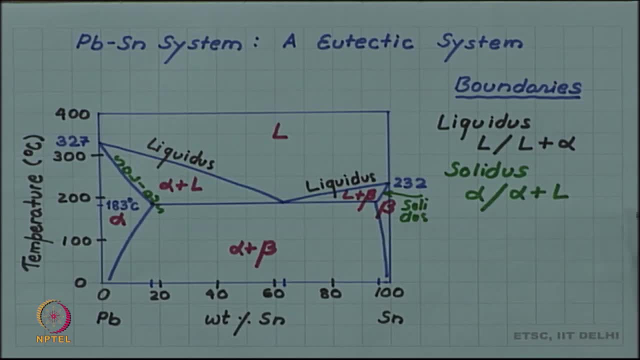 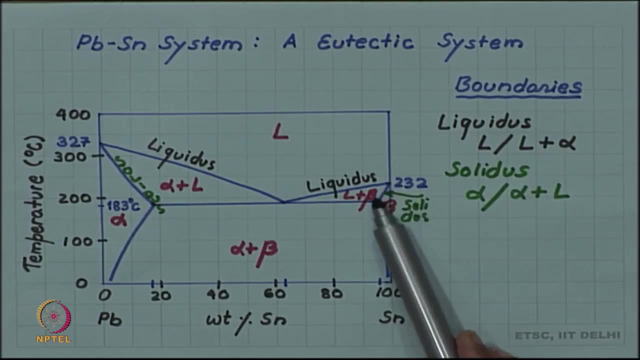 There also the same definition is valid, and when I say alpha, not necessarily that it has to be alpha. You can see here that this is a boundary between beta and liquid plus beta, and that is also solidus. So alpha represents any solid. So a solid with a boundary between a solid and the same solid plus liquid boundary will. 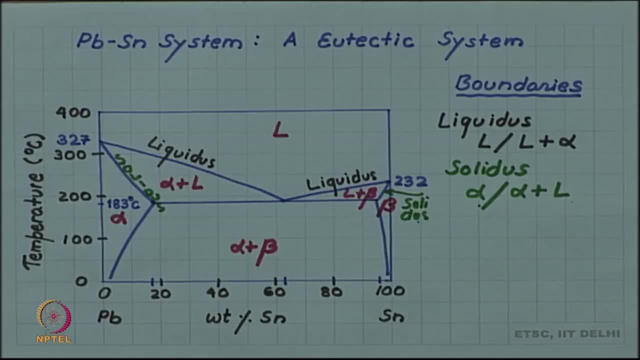 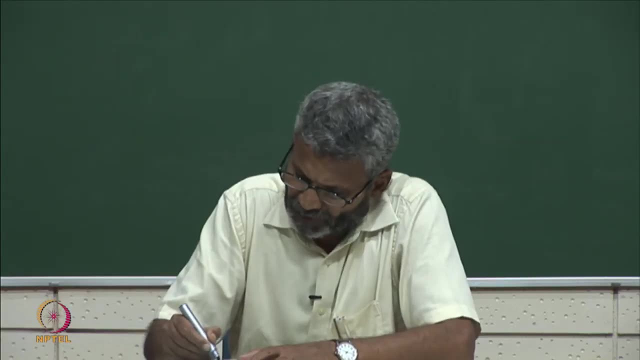 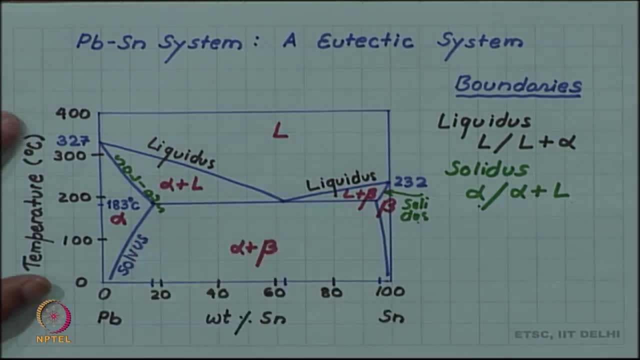 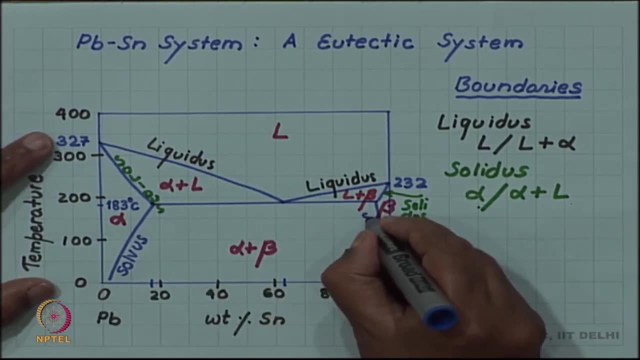 for the in comparison to the isomorphous system. They were not there because you had a single solid phase, but now you have two solid phases, So there are boundaries which are delineating that. these lines are called solvers. I have got this. 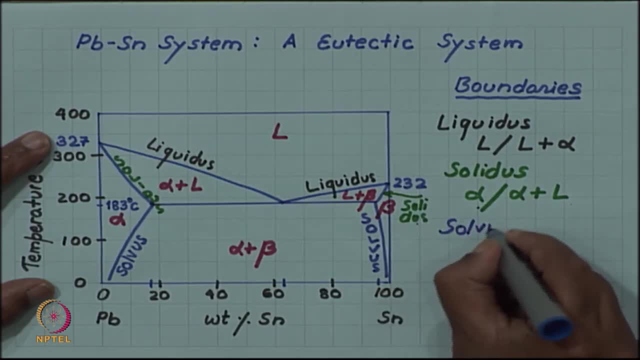 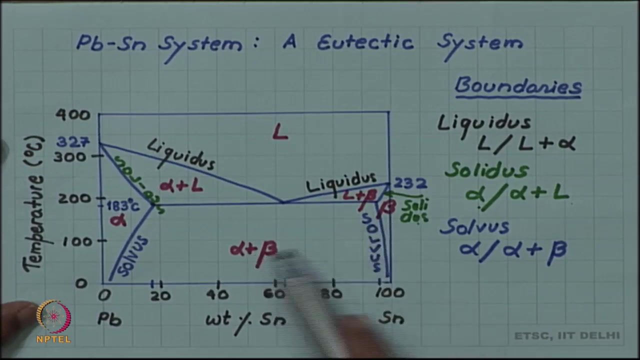 Thank you, Thank you, Thank you. So I have solvers, which is a boundary between a solid phase and then the mixture of two solids: alpha, alpha plus beta. Of course, beta, alpha plus beta is also another solvers. there, only one boundary is not yet. 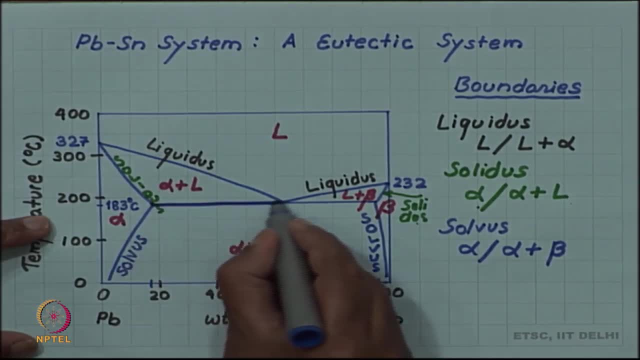 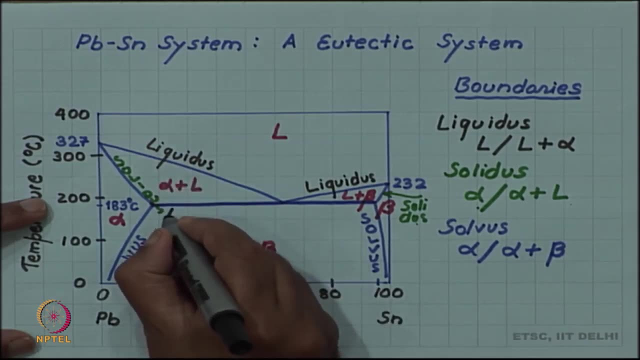 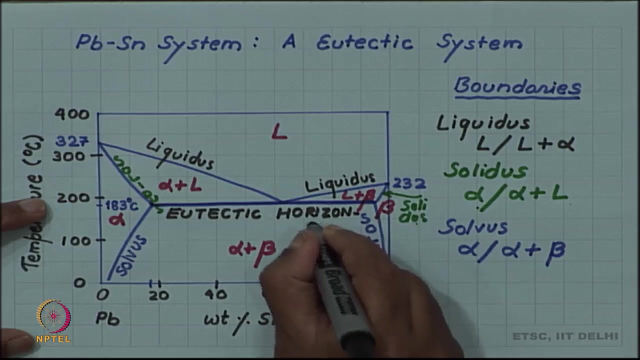 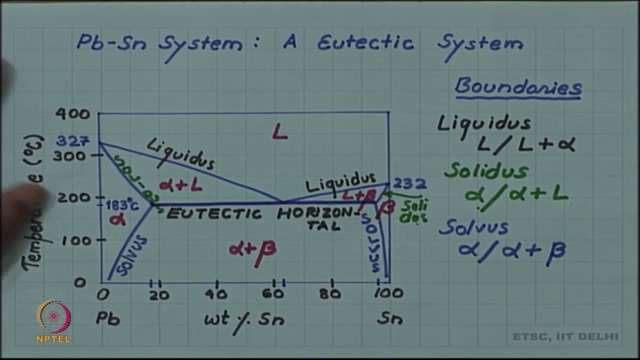 labeled and that is this horizontal line, which is a very important line in this diagram. Thank you. this we call the eutectic horizontal. So you have liquidus, you have solidus, you have solvus and you have eutectic horizontal. The name eutectic comes from the meaning of 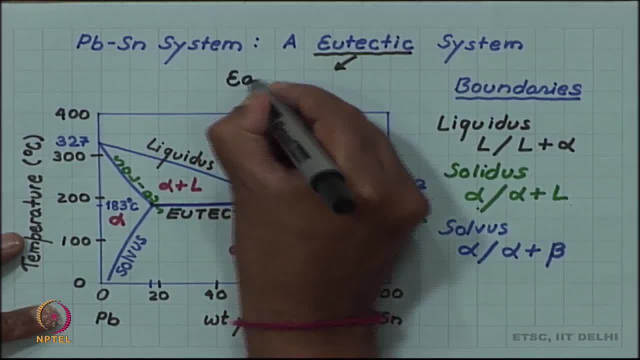 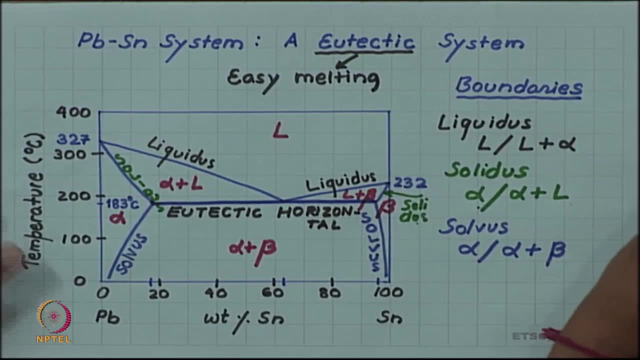 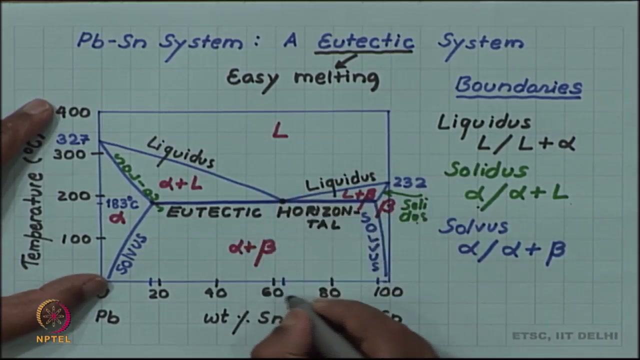 eutectic is easy melting. So in this alloy system there is one composition and that is the 62 weight percent tin. that is why I had started at 62, remember. So at 62 weight percent tin you have an alloy which will melt at a very low temperature. So if 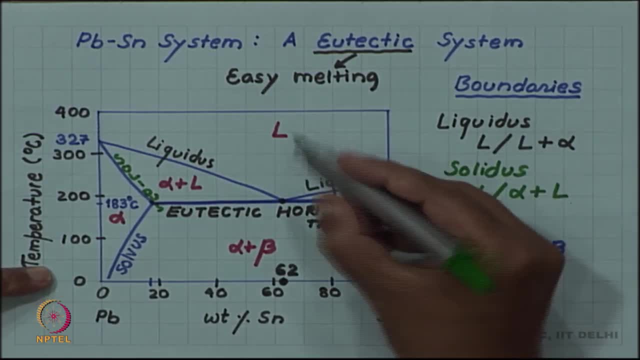 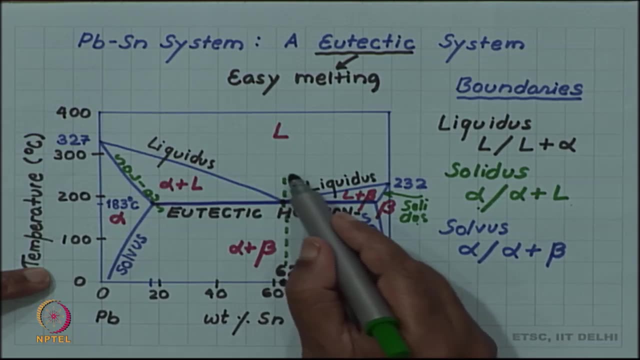 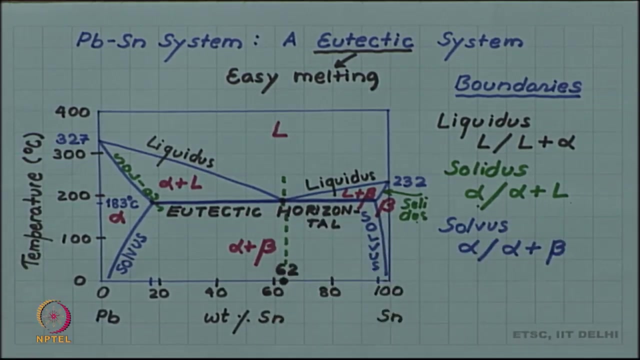 I take this alloy. if I draw the composition vertical at that alloy, you can see that this is liquid up to 183 degree Celsius and then it will become solid. So this alloy solidifies. although it is an alloy, it solidifies as a at a single temperature. 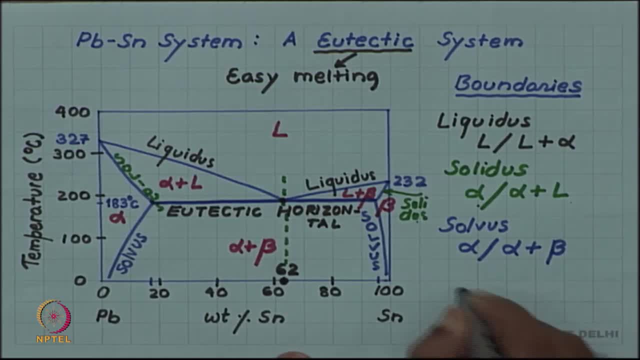 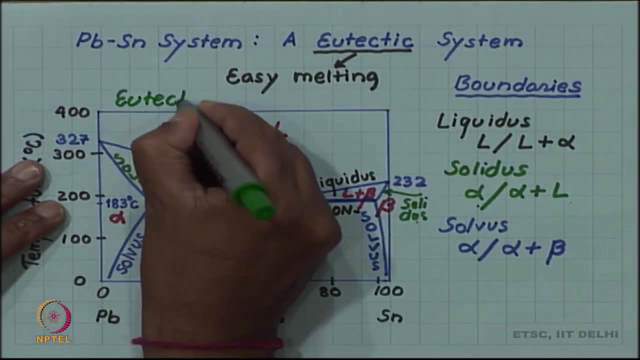 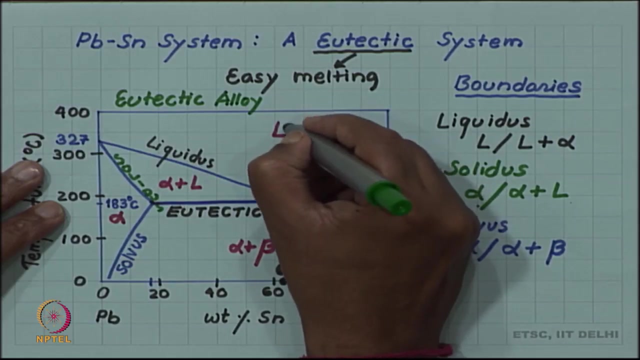 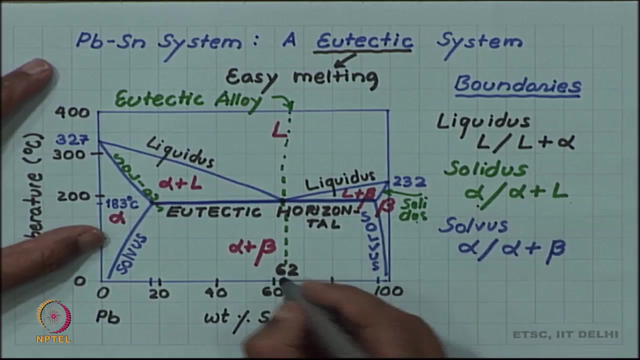 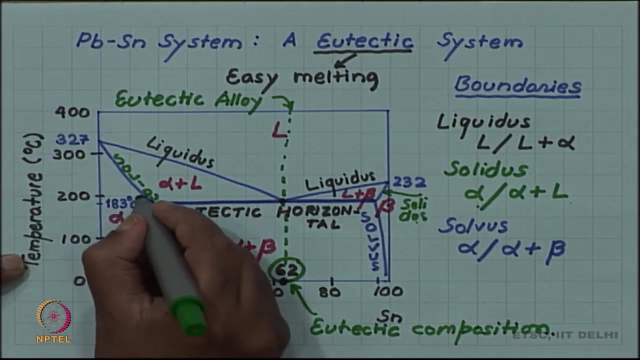 So this is specific alloy- is called a eutectic alloy. eutectic alloy, this particular vertical Ok Eutectic alloy, this composition, So correspondingly, this composition at which the eutectic alloy exist, this is called a eutectic composition. The temperature at which the eutectic alloy.